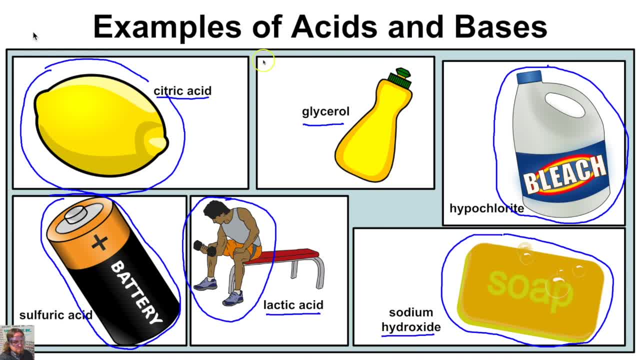 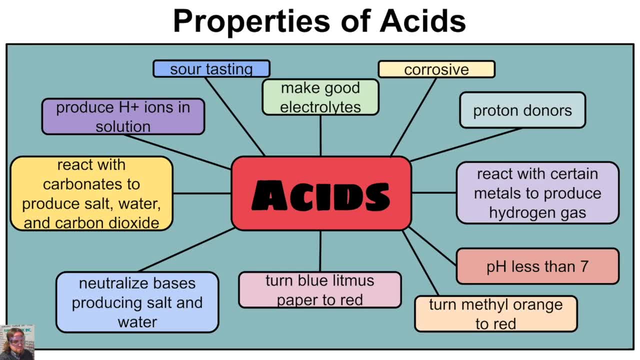 this is going to be a base. So some examples of acids and bases that you have had experience with before. Now let's take a look at some properties of acids and bases next. And so what are some properties of acids? Well, we know from prior experience that acids have a sour taste. For 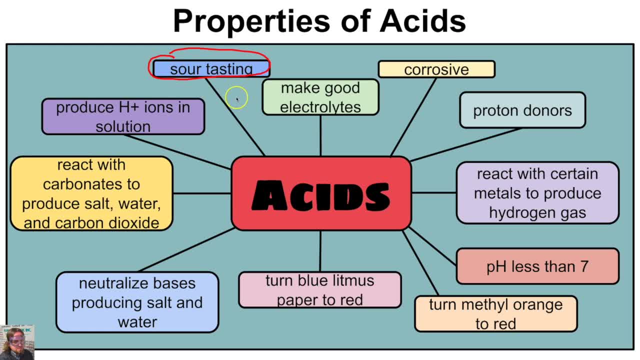 That lemon is going to have a sour taste due to the citric acid that is in it. We also know that acids conduct electricity. therefore they make good electrolytes. We know also that acids are corrosive. We know that acids can be proton donors. 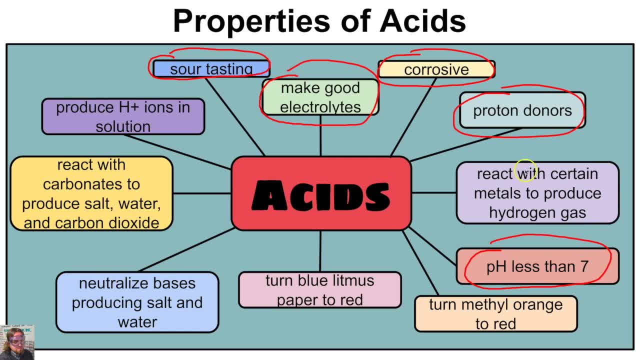 We know that acids have a pH of less than 7 on the pH scale. We also know that acids react with metals to produce hydrogen gas. Acids will also turn an indicator called methyl orange to red, and we'll talk about that later on in this little unit. 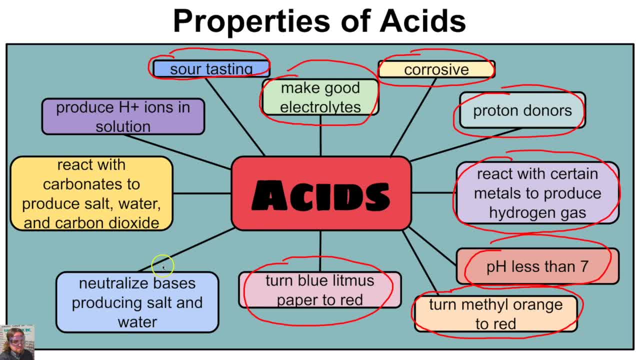 We also know that acids will turn blue litmus paper to red. Acids neutralize bases producing salt and water according to the Arrhenius model of acids and bases. Acids also produce H plus ions when dissolved in solution. Acids, last but not least, are going to react with carbonates to produce salt water and 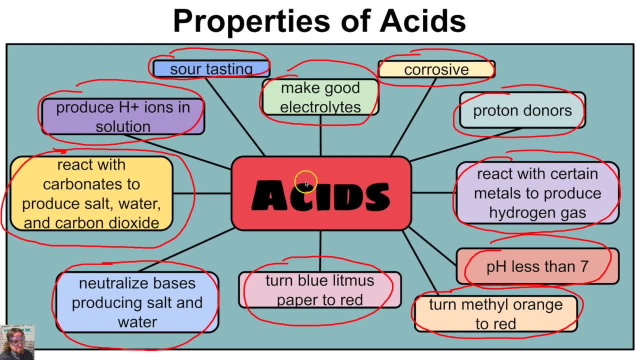 carbon dioxide. So these are some properties of acids and bases that you might or might not be familiar with, And if you are unfamiliar with some of these properties, we will learn about them in a future video. But now let's take a look at some properties of bases and then take a look at strong acids. 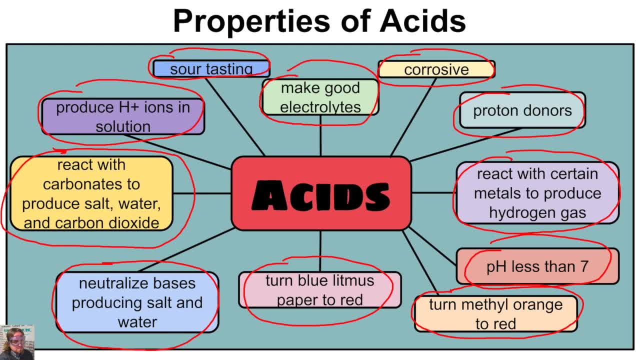 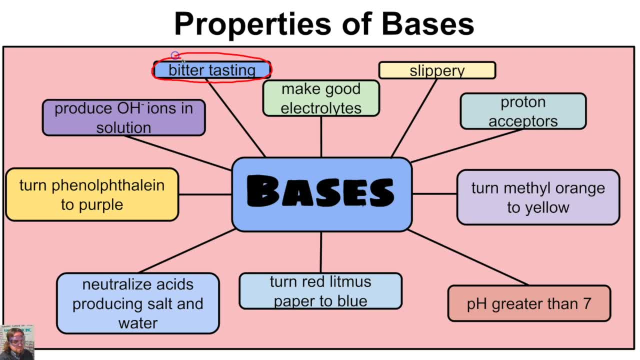 versus weak acids and strong acids versus weak bases. And so what are some properties of bases? Well, it says right here that bases have a bitter taste. If you bite into a bar of soap when you were a kid, maybe your mom washed your mouth out. 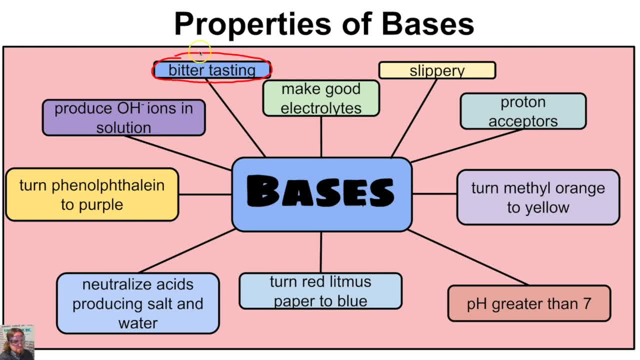 with soap. If you said a naughty word, well, that soap is going to have a bitter taste. We also know from prior experience That bases have a tendency to be slippery. If you've ever dropped the soap in the shower before, that's because bases are slippery. 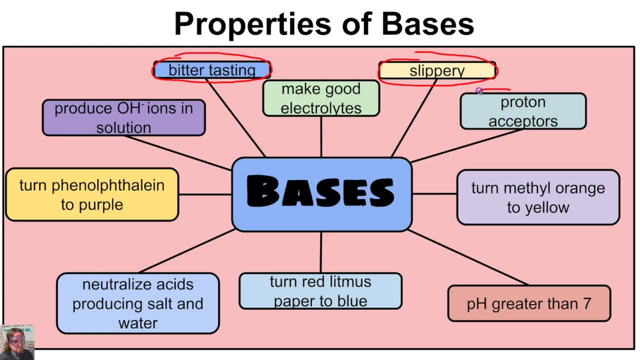 and soap is primarily a base or is going to be a base. We know that bases are going to be proton acceptors according to the Brunsted-Lowry model of acids and bases. we'll learn later on. Take a look at this. 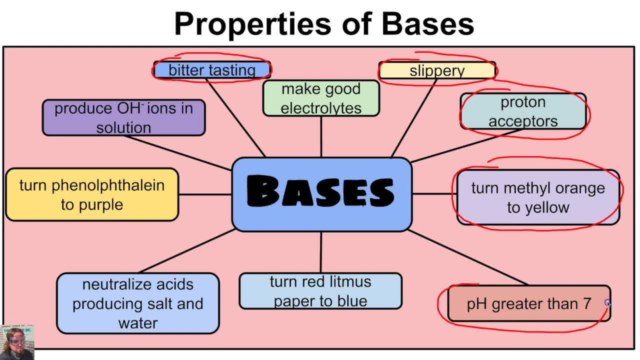 Bases are going to turn methyl. orange to yellow. Bases have a pH greater than seven. Bases turn red, litmus paper, blue. Bases neutralize acids producing salt and water, according to the Arrhenius model of acids and bases. 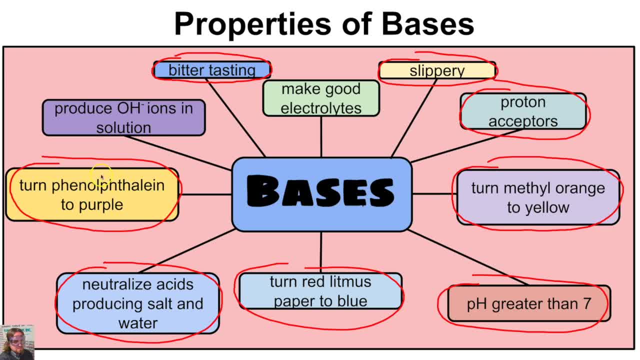 Bases also will turn phenolphthalein to purple, another type of indicator. we'll talk about this unit. And last but not least, bases are going to produce OH minus ions when dissolved in solution according to the Arrhenius model of acids and bases. 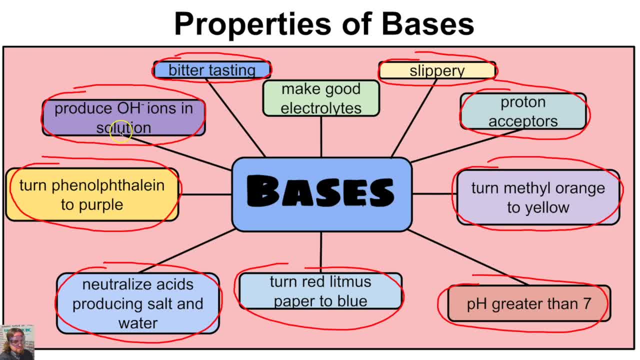 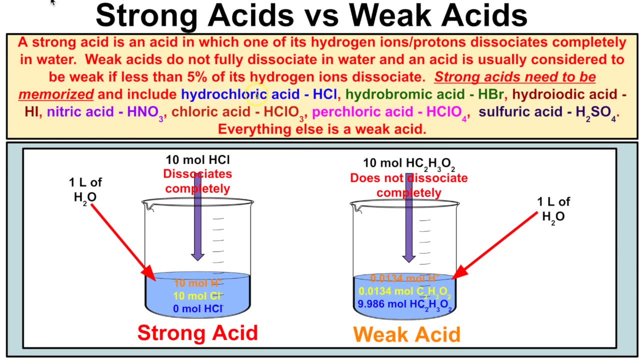 And so now let's take a look at some examples of strong acids and weak acids, and then take a look at some examples of strong bases and weak bases. And so what are strong acids and what are weak acids? Well, it says right here that a strong acid is an acid in which one of its hydrogen ions 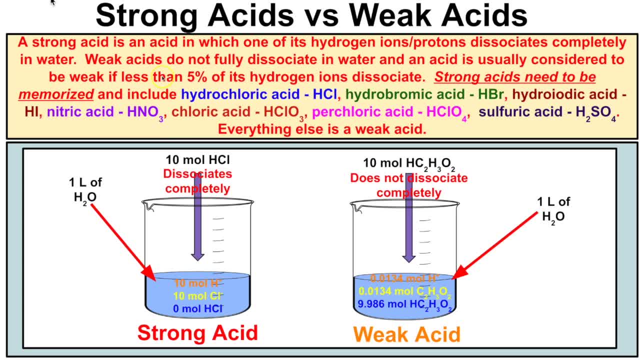 slash. protons dissociates completely in water, And weak acids do not fully dissociate in water, And an acid is usually considered to be weak if less than 5% of its hydrogen ions dissociates. So what does this mean? Well, let's take a look right here. 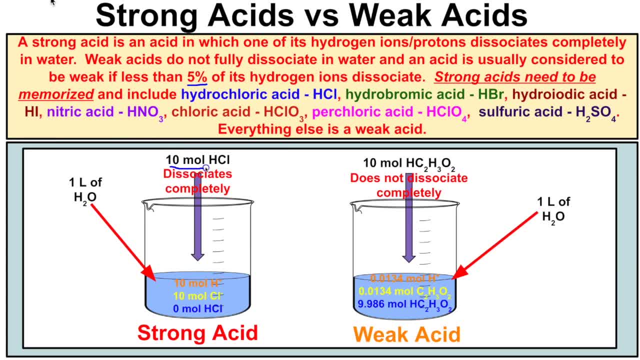 We have a beaker of water, And what does this mean? Well, let's take a look right here. We have a beaker of water, And what does this mean? So what we're going to do is we're going to place 10 moles of HCl in this beaker of. 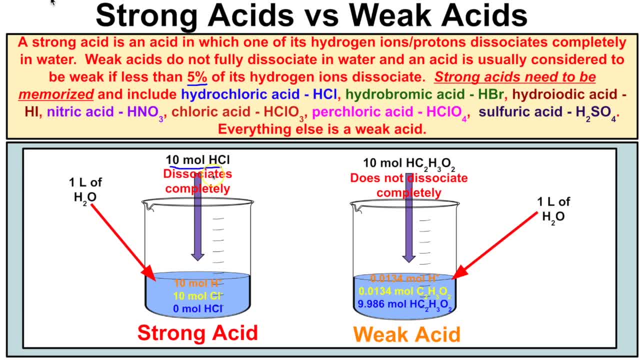 water. And when we do that, what ends up happening is that this 10 moles of HCl is going to dissociate completely. It's going to break apart and form 10 moles of H plus and 10 moles of Cl minus here and 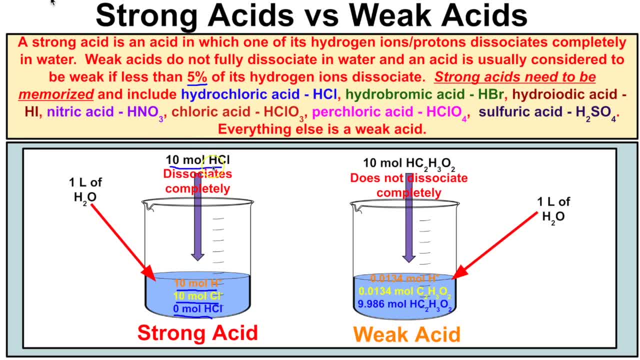 no moles of HCl. So this entire 10 moles of HCl is going to dissociate and break apart into 10 moles of H plus and 10 moles of Cl minus. So, because of this, HCl or hydrochloric acid is going to dissociate. 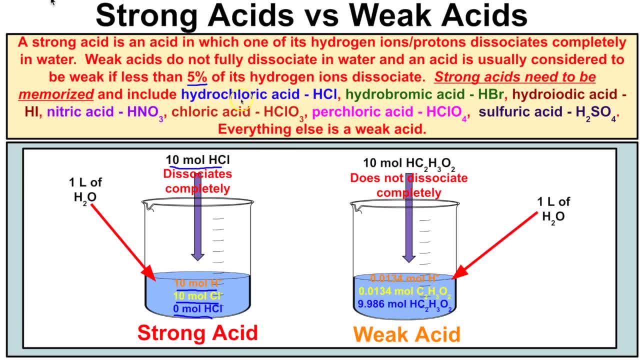 And that's because HCl is considered to be a strong acid, And so there are about seven strong acids in chemistry And all other acids are going to be weak acids, And so if you simply memorize the list of seven strong acids, you should be good. 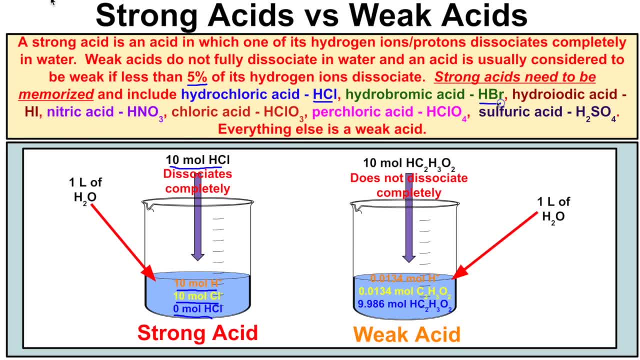 The seven strong acids are: hydrochloric acid, or HCl, hydrobromic acid or HBr. hydroiodic acid, or simply HI. nitric acid, which is HNO3,. chloric acid, which is HClO3,. 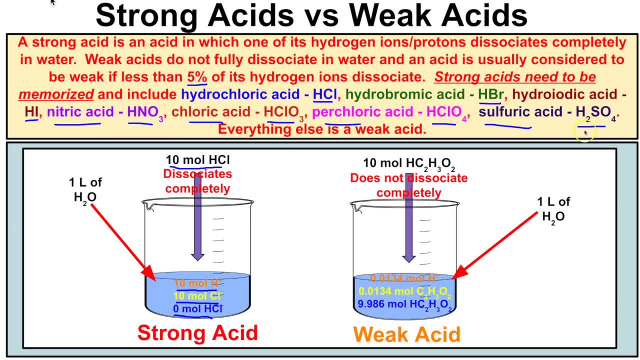 perchloric acid, which is HCl4, and sulfuric acid, which is HCl2.. acid which is H2SO4. so everything else is going to be a weak acid. so what is a weak acid? well, let's suppose we have 10 moles of this stuff right here, HC2H3O2, and we put this in water right here. 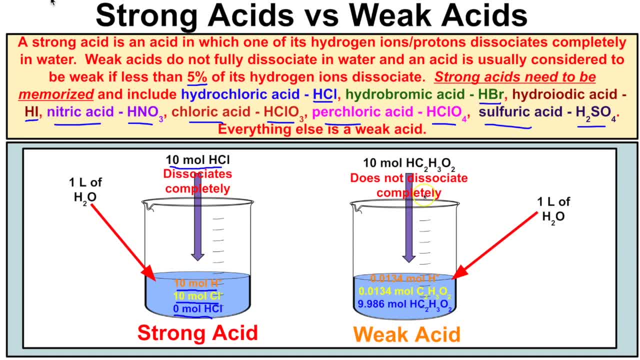 well, as we see right here, this is not going to completely dissociate. in fact, if we take a look, if we put 10 moles of this stuff in here, we're going to end up with 9.986 moles of this substance still floating around in this water here. it is not going to dissociate, it is not going to break. 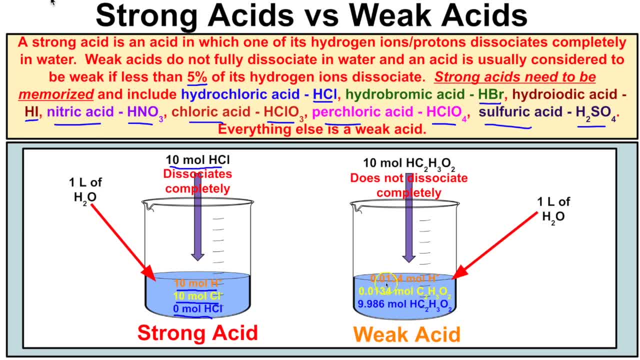 apart and we're only going to end up with about 0.0134 moles of H plus and 0.0134 moles of C2H3O2, and so understand that concept that a strong acid is going to completely dissociate and break apart. 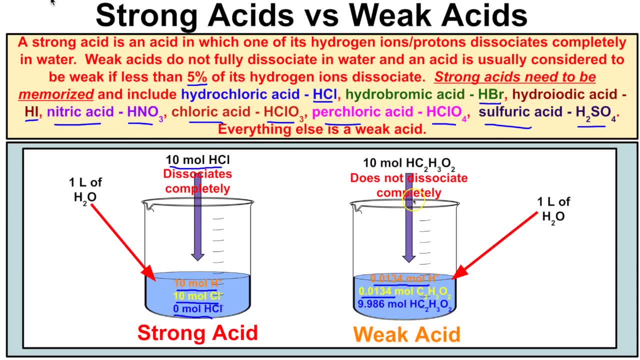 where a weak acid is not going to completely dissociate. in fact, it's not going to dissociate much of much at all, and so we're going to have relatively low amounts of H plus ions floating around in this weak acid and a relatively high amount of H plus ions floating. 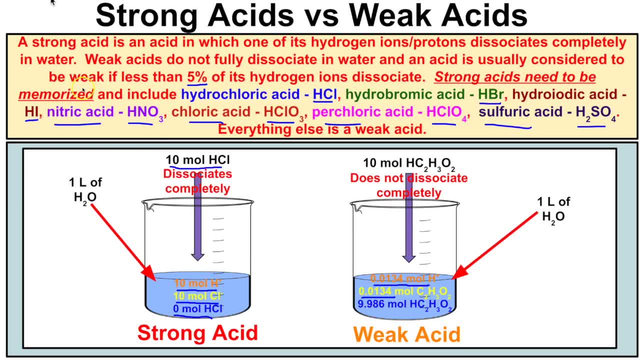 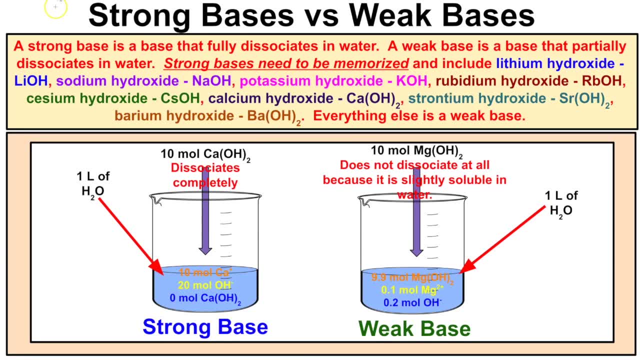 around in this strong acid right here. so now let's take a look at strong bases versus weak bases. and so it says right here that a strong base is a base that fully dissociates in water. and so if we take a look once again, let's suppose we have 10 moles of this substance here: calcium hydroxide. 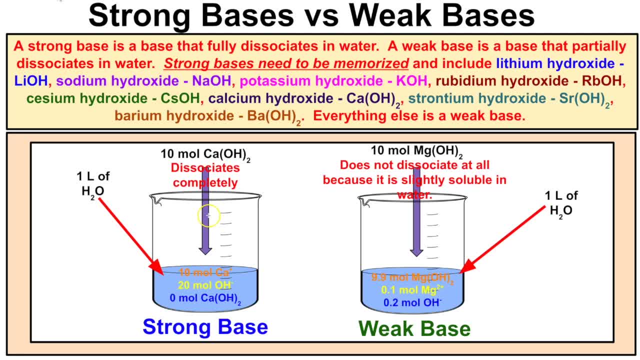 and when we put this in water, it's going to completely dissociate. and so, if this completely dissociates, what we're going to end up in this water with is 10 moles of calcium ions and 20 moles of OH, minus ions floating around in this water right here, and so we're not going to have any moles of calcium. 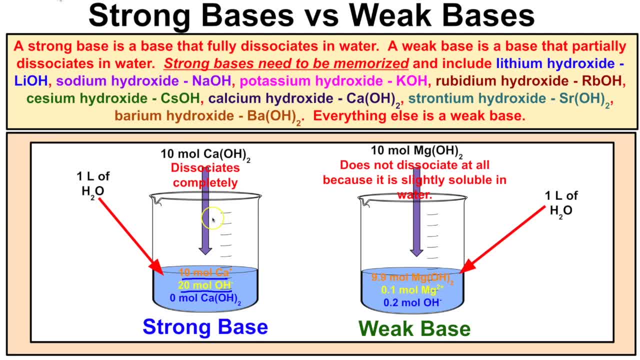 hydroxide, because it's going to completely dissociate, it's going to completely break apart, and so calcium hydroxide here is considered a strong base for this reason, and so here's a list of strong bases that you need to memorize, and everything else is a weak base. make sure you 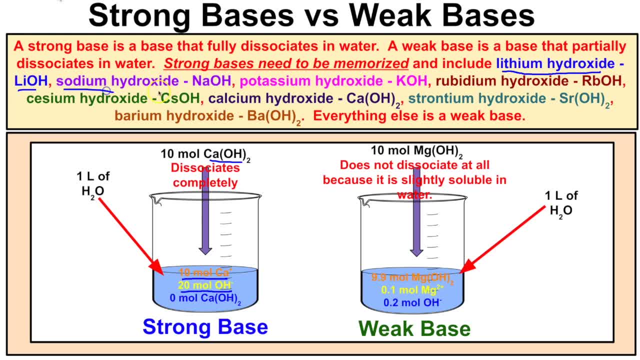 memorize list of strong bases that you need to memorize and everything else is a weak base. the two bases that we're going to be using today, like potassium hydroxide or LiOH, sodium hydroxide or NaOH, potassium hydroxide or koH rubidium hydroxide, rboh, cesium hydroxide and 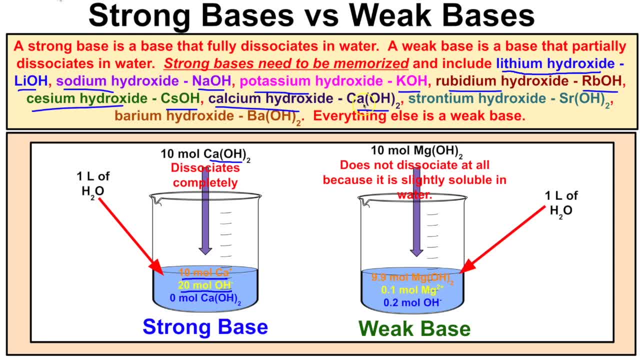 C, SOH and calcium hydroxide as your strong bases, as well as strontium hydroxide and barium hydroxide as well. so these are going to be your strong bases and everything else is going to end up being a weak base. and if we take a look at a weak base, let's suppose we have ten moles of 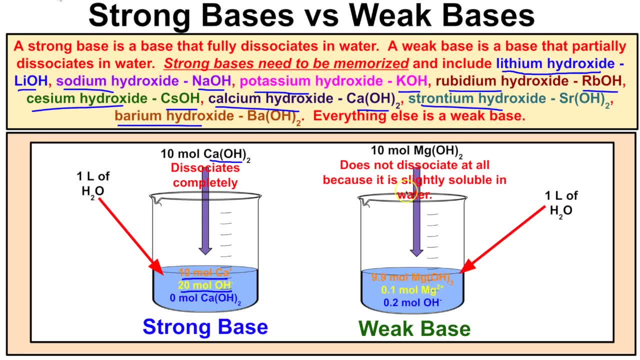 magnesium hydroxide. these are solid bases, these are beyond that. so you can imagine right here this: well, if we put this in water here, this substance right here is slightly soluble in water and so it's not completely soluble in water. not all of this is going to even dissolve, and so, if not all, 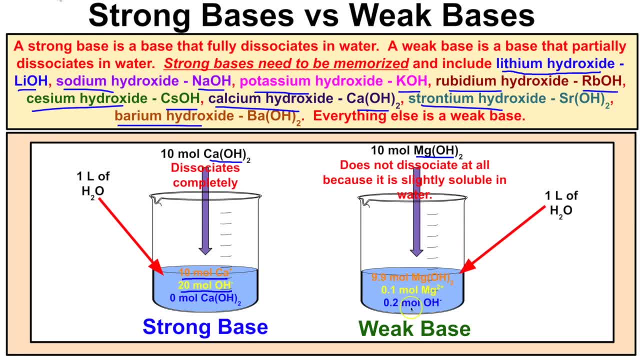 of this dissolves, then you're not going to have very many OH minus ions floating around in this solution right here and this is going to end up being a weak base. so understand that concept where strong bases completely dissociate in water and weak bases do not fully dissociate in water and 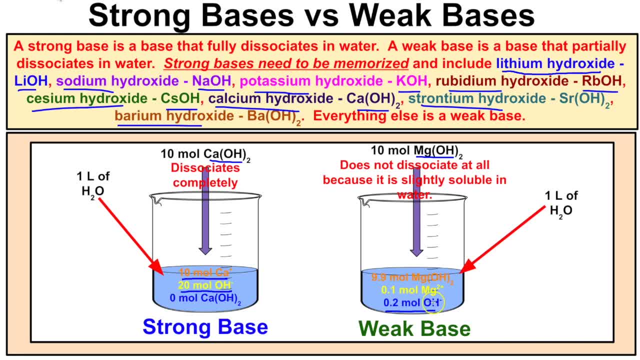 you're going to have a relatively low amount of OH minus ions that are floating around in this, in this beaker of water right here. all right, so that's properties of acids and bases. understand what some of those properties of acids and bases are. make sure you understand what. how strong acids. 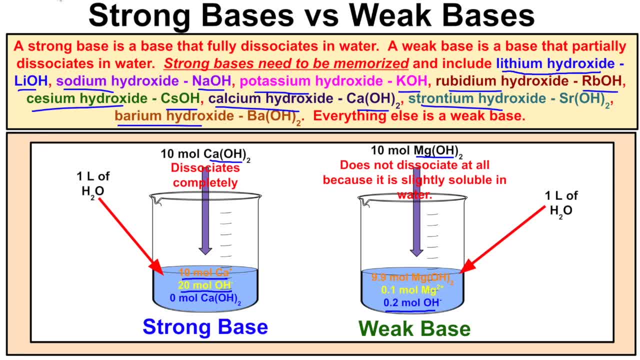 versus weak acids work and strong bases versus weak bases. and if you like this video, please subscribe to my channel and hit the bell icon so you don't miss any of my new videos, and I'll see you in the next video. Bye, like what you see, go ahead and click that little bomb in the bottom right hand corner. that's going. 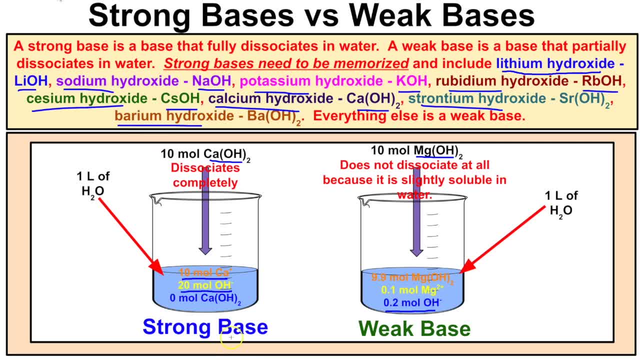 to subscribe to my channel and feel free to leave any comments or questions down in the comment section down below, and I really hope you guys found this helpful.